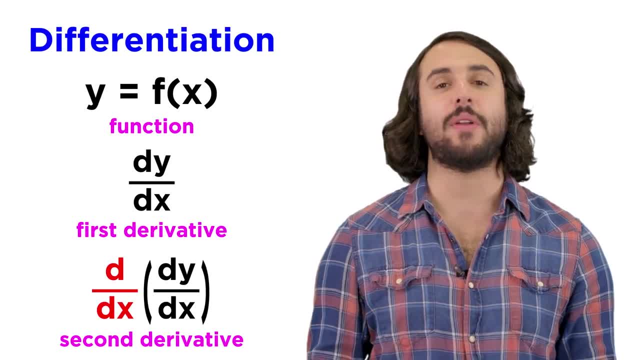 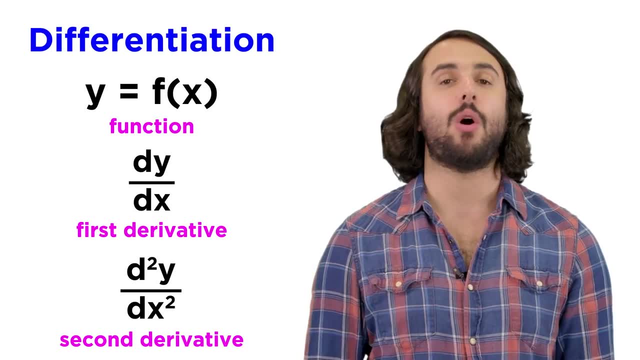 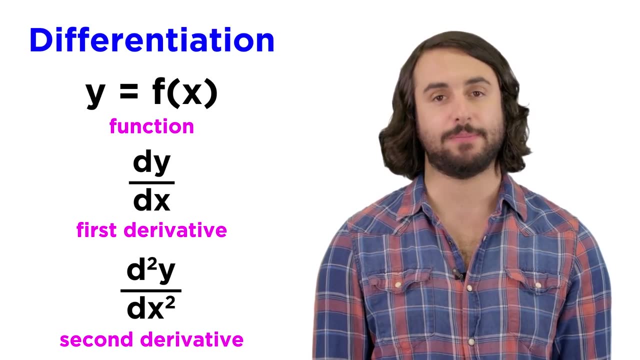 that that would be dy over dx. So if we take the derivative of that by placing d over dx out here, that can be represented as d squared, y over dx squared. So this notation also indicates a second derivative, just like f double prime. 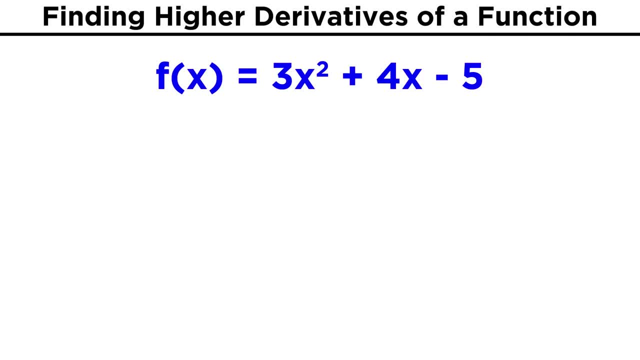 For simple polynomials, finding the second derivative is not hard to do at all. Take three x squared plus four x minus five. Taking the derivative of this by using the power rule, we get six x plus four as the first derivative. and then we just take the derivative of this to get six as the second. 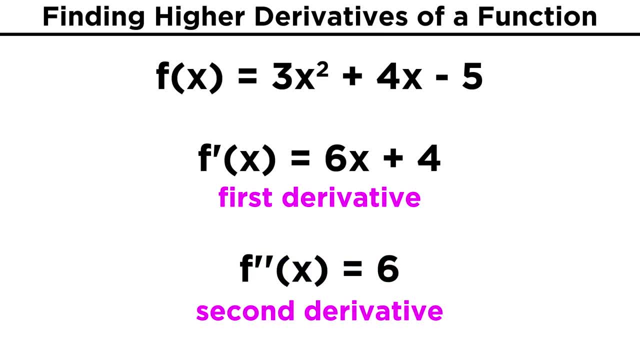 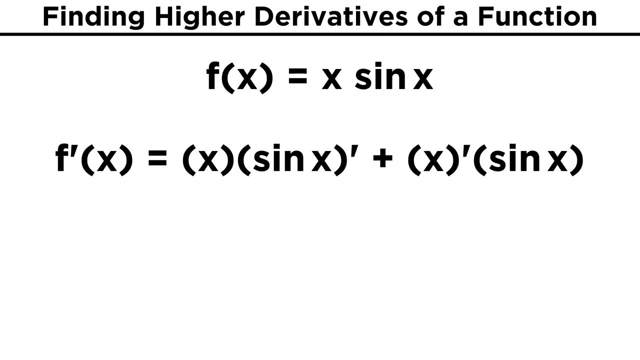 derivative. All we did was take the derivative twice. Of course, this could get a little trickier. Take x sine x. To get the first derivative we need the product rule. so, remembering how that works from a previous tutorial, Let's take the two functions where they go and take these two derivatives. 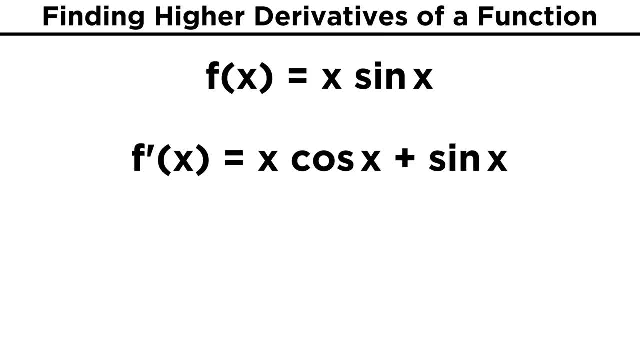 We should get x, cosine x plus sine x. Then to get the second derivative, we just take the derivative of this new function For the first term. again, we need the product rule. so we set it up just as we are used to and evaluate the derivatives. 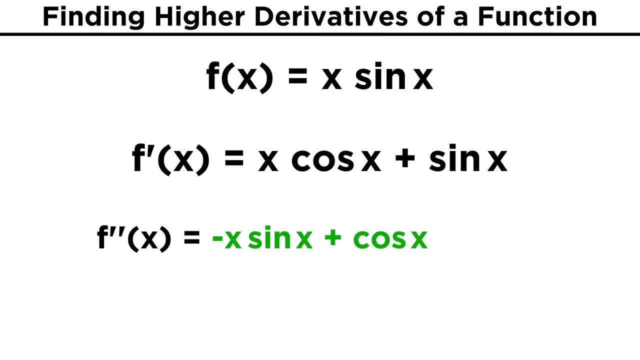 That should give us negative x sine x plus cosine x. And then we can't forget this derivative, We can't forget this other term here, which simply becomes cosine x. So that gives us negative x sine x plus two cosine x as our answer. 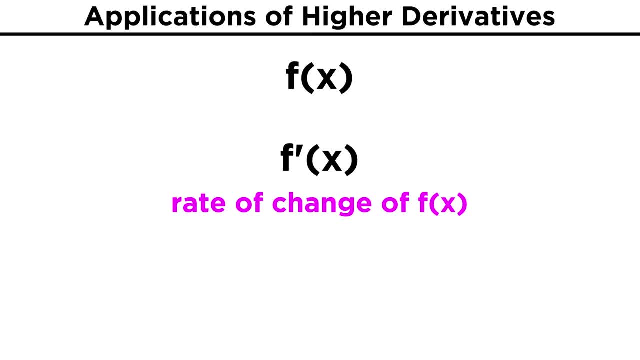 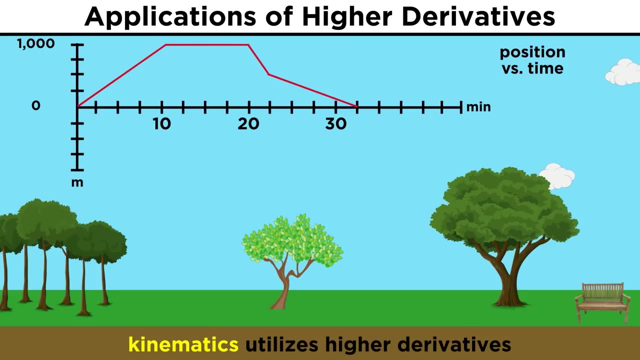 So why is this useful? Well, let's recall that a derivative represents the rate of change of a function. This means that a second derivative represents the rate of change of the rate of change of the function. That may sound confusing, But there is an extremely good use for this in kinematics, the study of motion, which 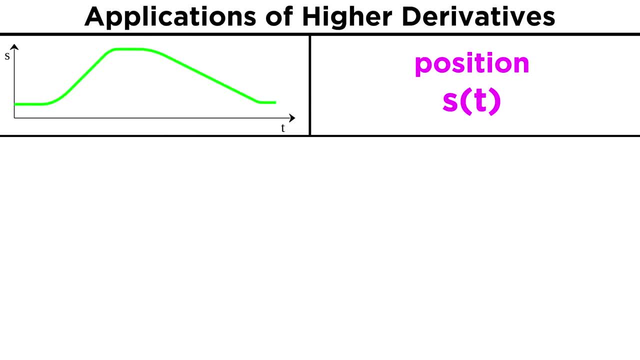 we covered in the classical physics course, We can make a graph of the position of an object versus time. This could be a falling object, a speeding car, pretty much anything. As we've mentioned before, the derivative of this position function will be the rate. 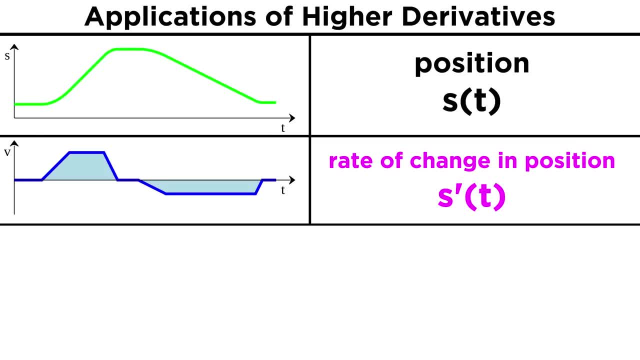 of change in the function or the change in position with respect to time, And that's velocity. So velocity is the derivative of position, But the derivative of this velocity function will be the change in velocity with respect to time, and that's acceleration. 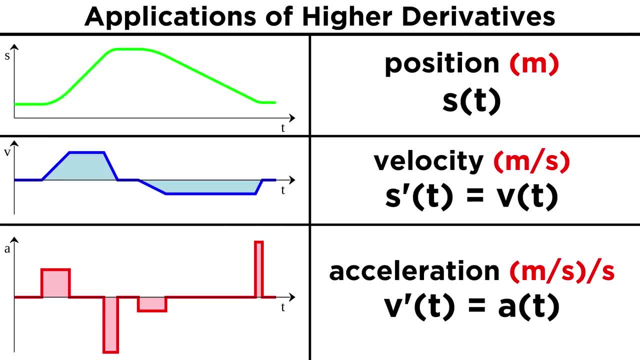 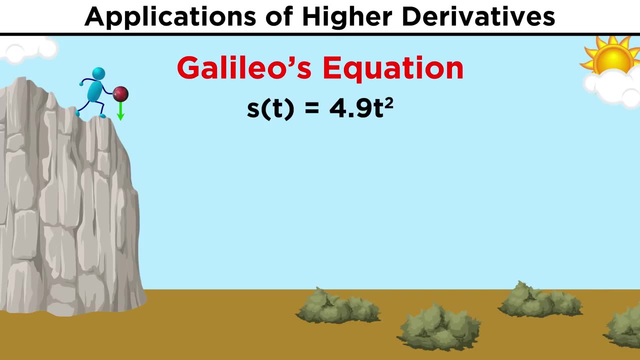 Position is meters, velocity is meters per second and acceleration is meters per second per second or meters per second squared. That means that acceleration is the second derivative of position and that A of t equals V prime of t. This is one way of understanding the acceleration due to gravity on Earth, as it relates to Galileo's 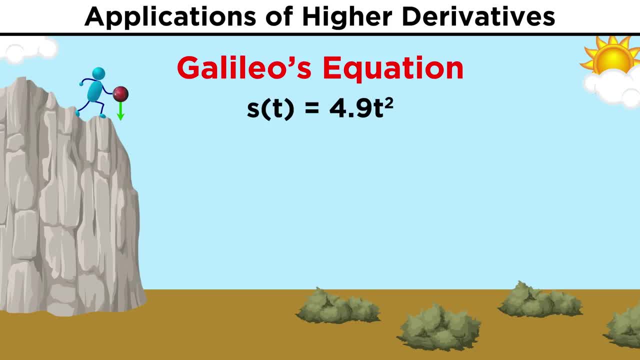 law for the position of an object in freefall. He derived the equation four point nine t squared by observation, and if we take the derivative of this we get nine point eight t. And if we take the derivative of that we get nine point eight. and this is why acceleration. 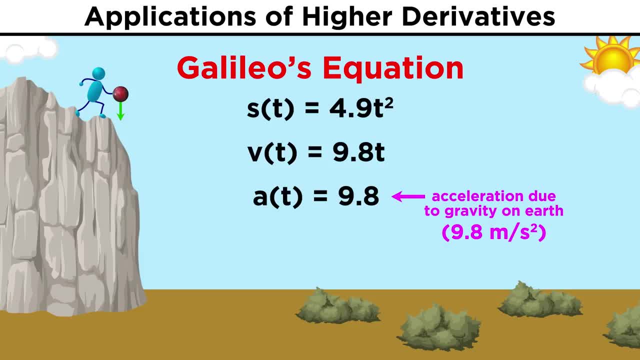 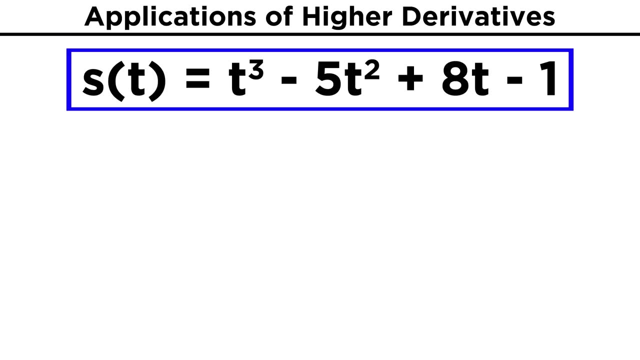 due to gravity on Earth is a constant equal to nine point eight meters per second squared. This understanding makes it extremely simple to answer questions in physics that would be tedious without calculus. For example, say: we have this function, S of t, that represents the position of an object. 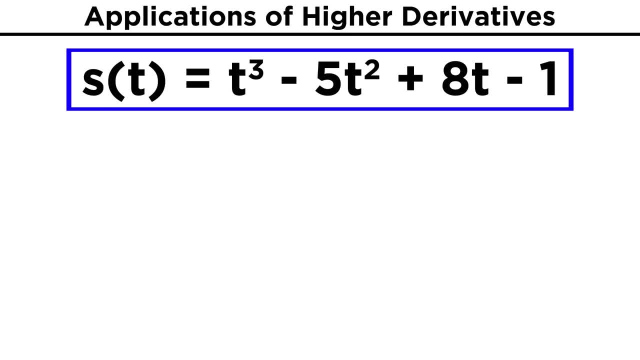 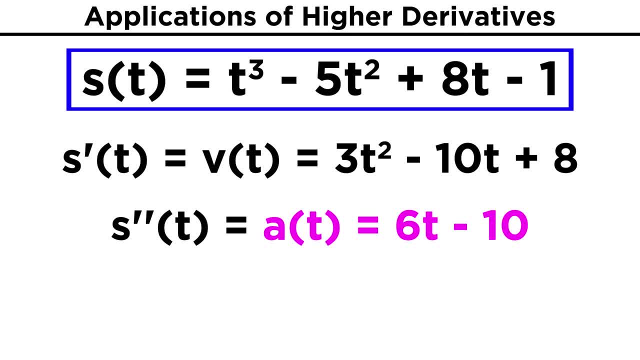 Since this represents the acceleration at any time. t, then, to find the acceleration at precisely five seconds, we just plug in five. A of five will be six times five, or thirty minus ten, which is twenty meters per second squared. Now, although we won't go beyond the second derivative all that often, there is nothing.